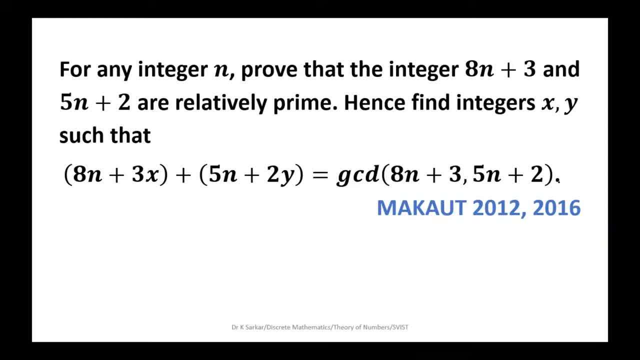 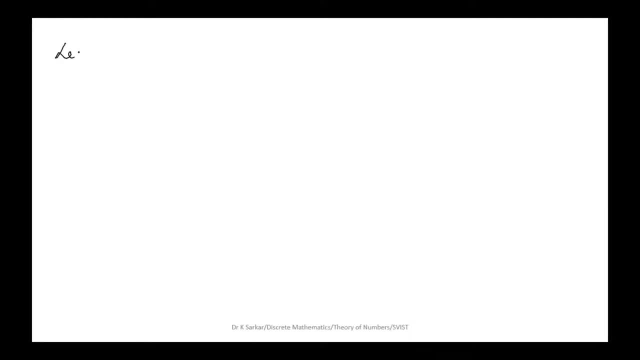 5n plus 2.. This question has appeared in Mac held 2012 and 2016 type. Let a equal a10 plus 3, and b equal 5n plus 2.. From this relation, we will have: n equals to a minus 3 by 8.. 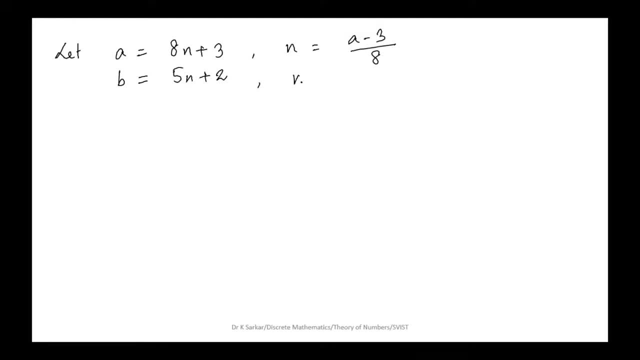 And from this equation, n as equal to a plus 3.. And from this equation, we will have n as equal to x as a minus 3 by 8.. we will have n equals to b minus 2 by 5. both of them are equal to n, so we can write a minus 3. 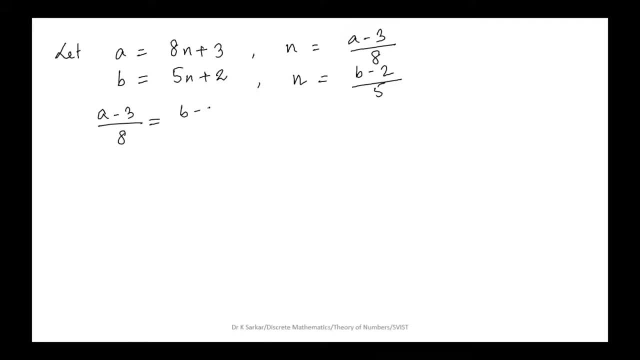 by 8 equal b minus 2 by 5, which imply 5a plus 8b. so in left hand side it is minus 8. b equal 16 minus 15, that is 1. so this imply a and b are prime to each other. 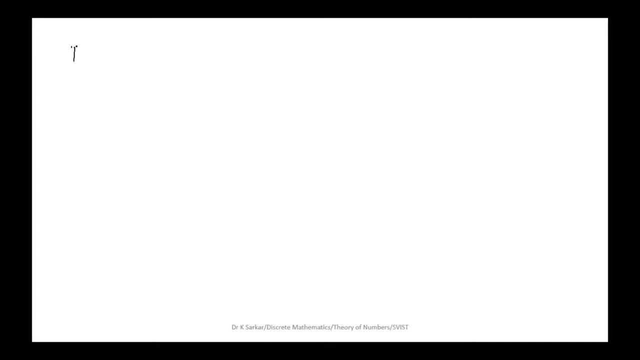 because we know this theorem: if a and b be integers, not both zero, then a and b are prime to each other, because we know this theorem. if a and b be integers, not both zero, then a and b are prime to each other. because we know this theorem: if a and b be integers, not both zero, then a and b are prime to each other. 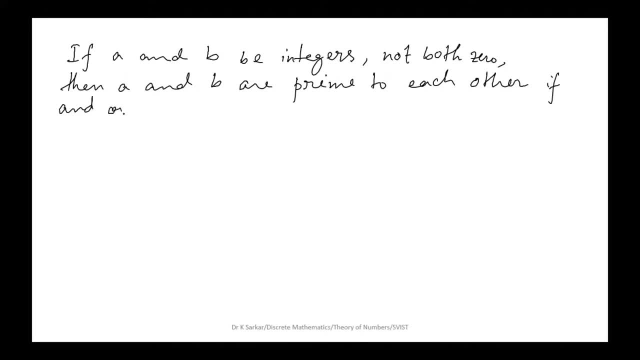 if, and only if, there exist integers u and v such that such that a u plus b v equal 1. therefore gcd of av equal 1. now, what is a 18 plus 3? what is b 5n plus 2? so gcd of 18 plus 3. 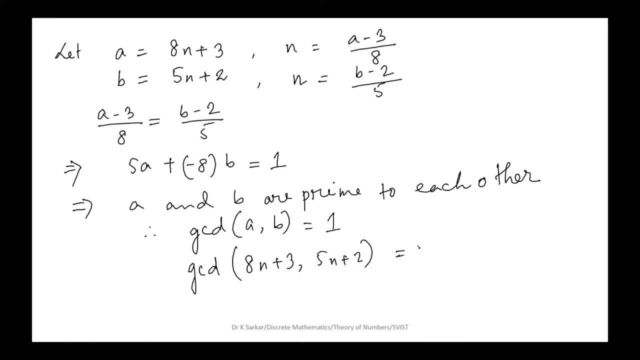 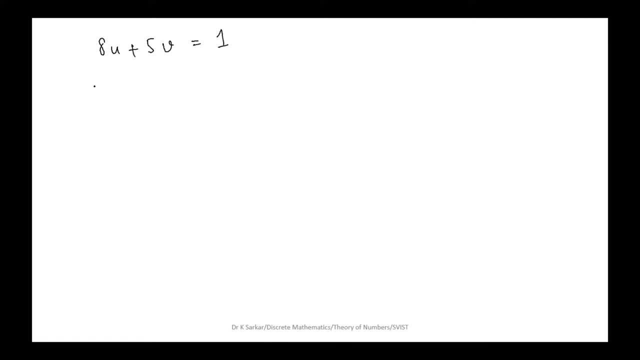 5v, equal 1.. Now what is given in the question? given that 8n plus 3x plus 5n plus 2y, equal gcd of 8n plus 3 comma, 5n plus 2.. Therefore, 8n plus 3x plus 5n plus 2y, that is equal 1..